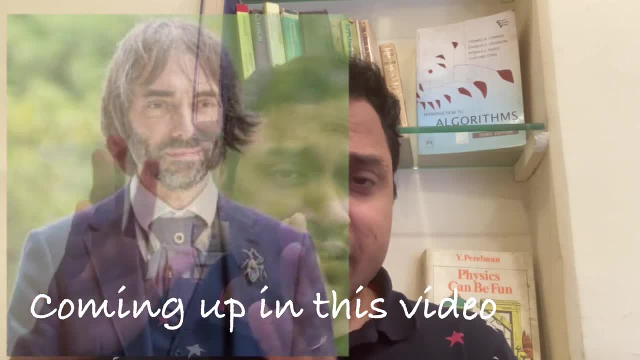 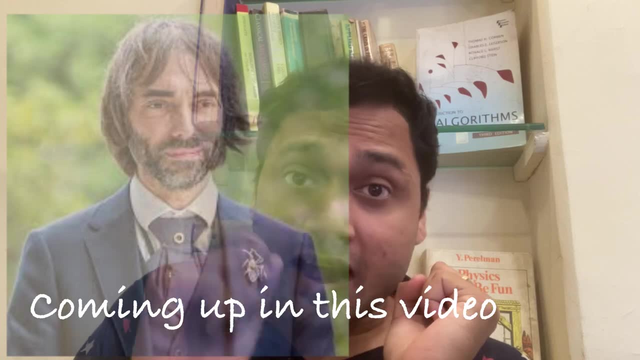 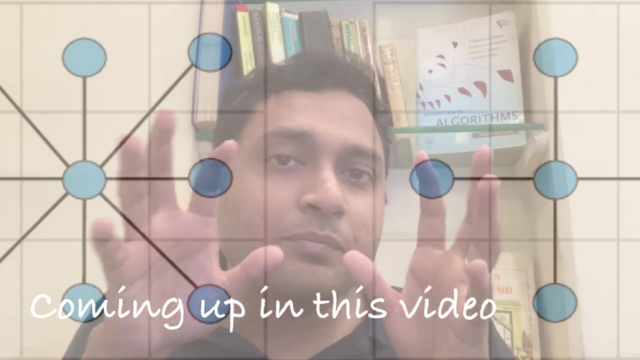 mathematicians of our time. Cedric Villani created a very beautiful investigation on how to teach mathematics at elementary school level, and one of his recommendation was to do hands-on mathematics. Adjacency relation is a very important relation, In fact, relations themselves. 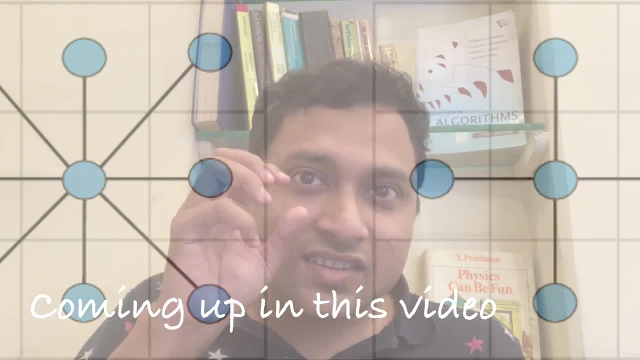 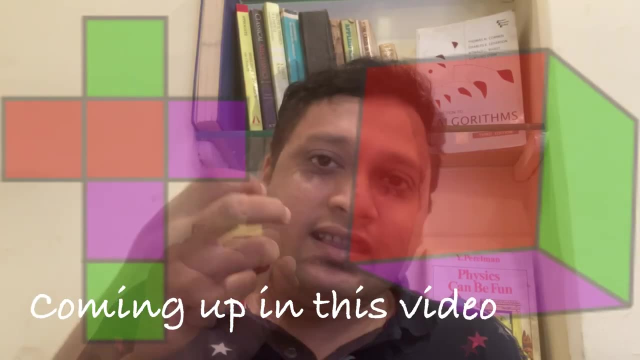 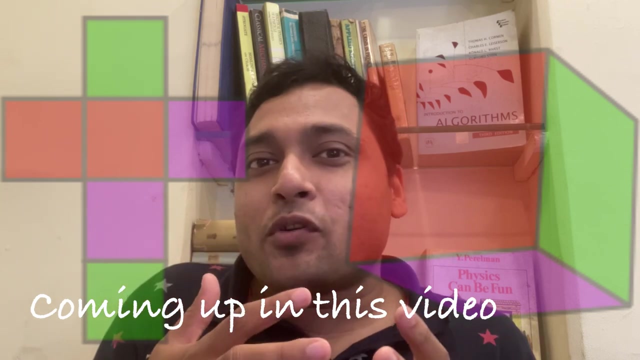 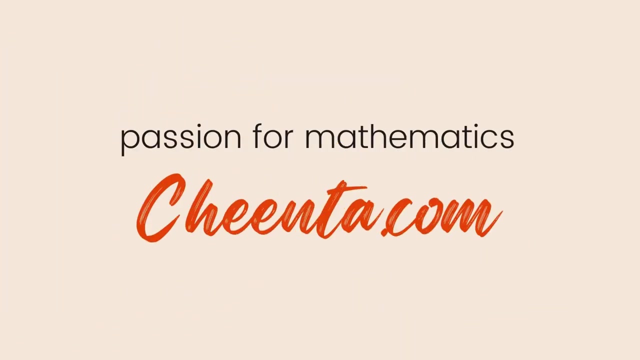 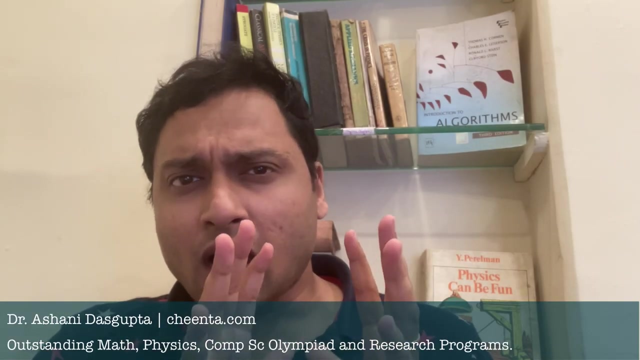 are quite important. It's very intuitive and structured in nature to understand relations. It's sort of the first step toward understanding structured knowledge. They sort of grasped the idea pretty quickly and then we could actually propose more complex problems. One of the things that is really close to my heart is how to introduce mathematics to children. 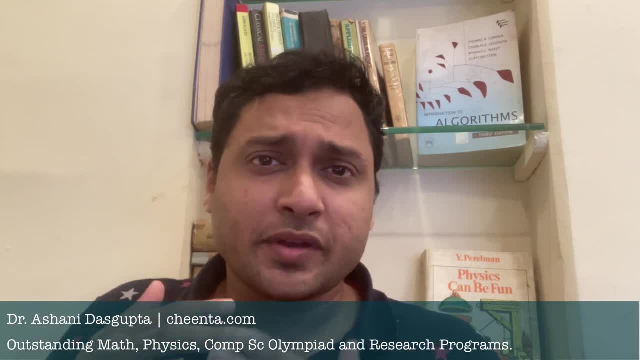 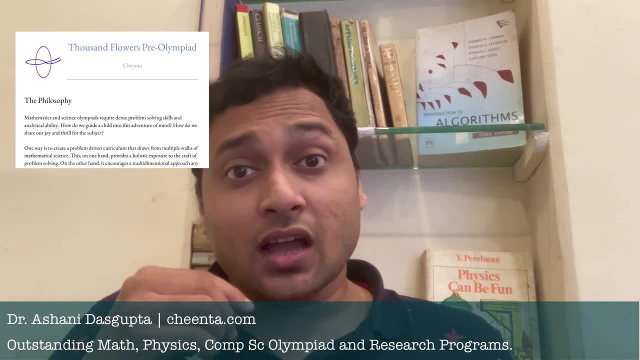 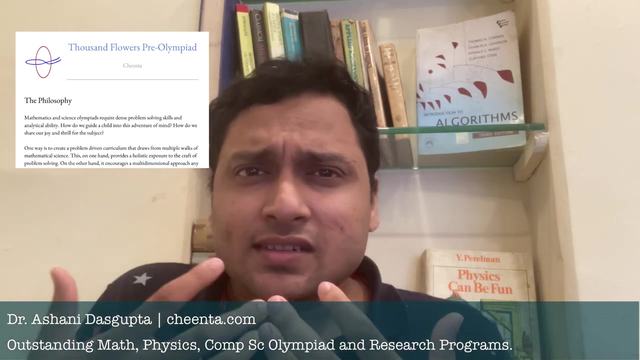 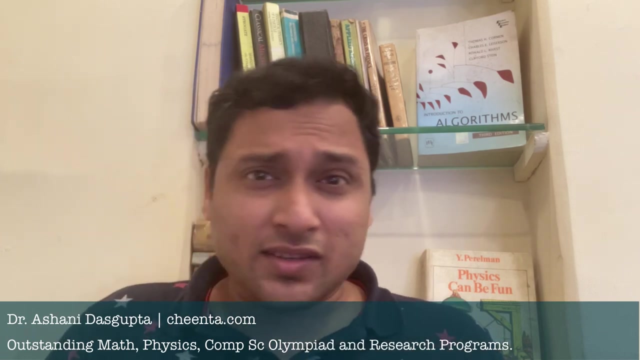 Children means elementary school students, students of grade one through four. Now perhaps you already know this, Chinta has something called the thousand flower programs, Math Olympiad programs for young kids, And we are constantly reviewing and innovating in that sphere of mathematical training because it's very sensitive. We learn a lot from 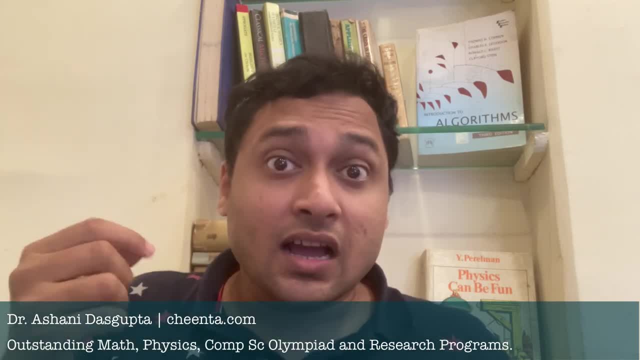 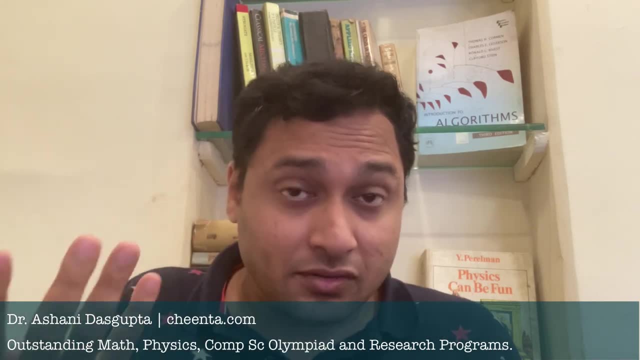 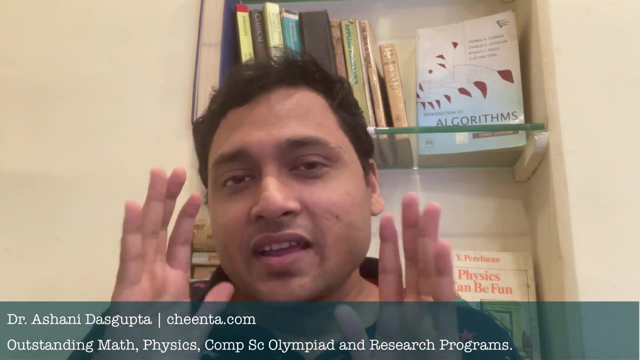 the kids over the last 10 years. We have learned how kids learn and it's an ongoing process. We cannot claim that we have already learned everything that is there to learn. In fact, I think we are only 10 or 20 percent on that way. But what we really believe is that people who are at the higher 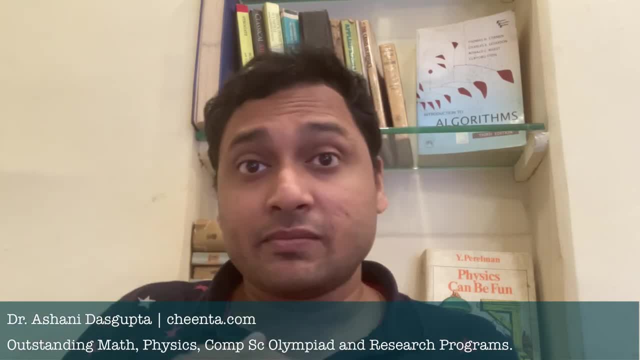 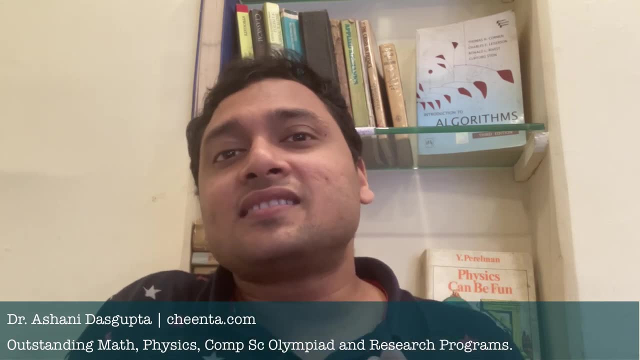 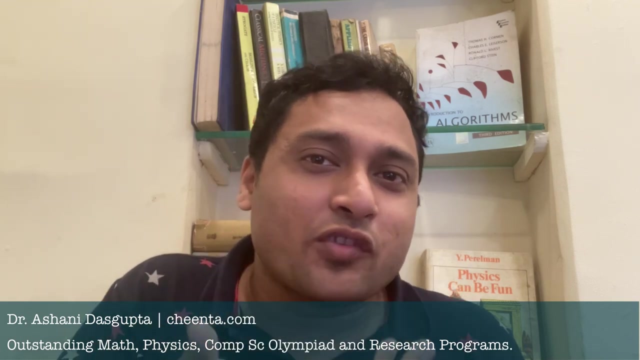 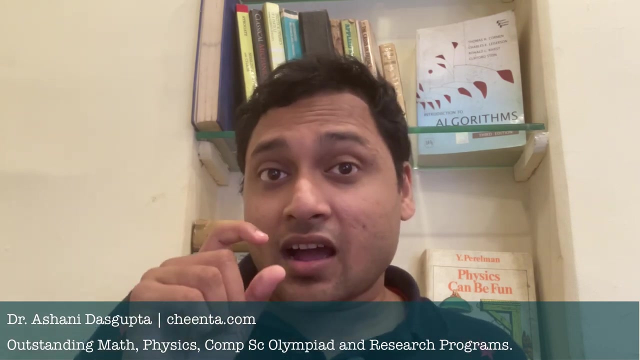 stages of mathematics, maybe who are doing university mathematics, who are doing research mathematics and who are interested to teach. they should invest serious time in creating curriculums, creating problems that are helpful for elementary school students, And that's exactly what we are doing here. It's a very hard job because children are most sensitive at that. 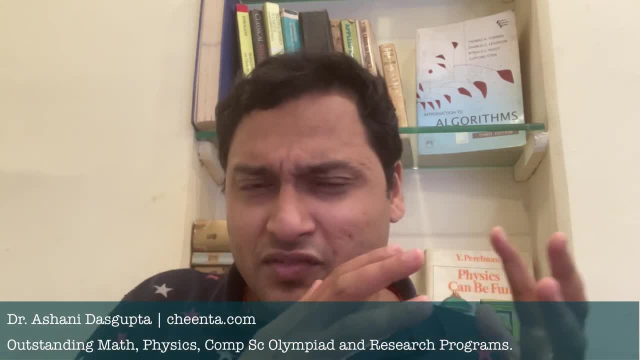 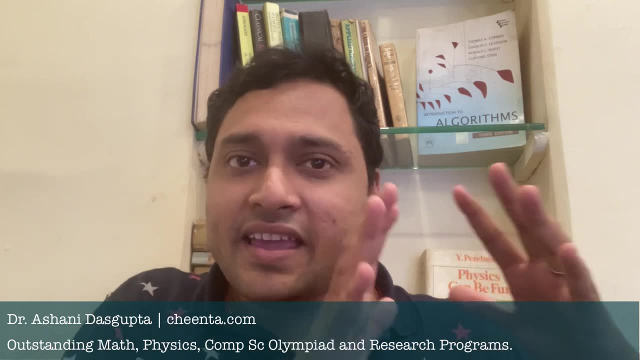 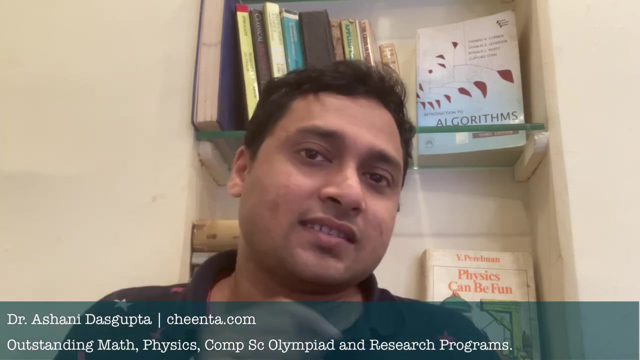 particular age and their brains are sort of taking shape. the neural pathways are making their own way, So it's very, very sensitive age span in their life. Today I want to talk to you about one such experience that we have had in this particular program and what 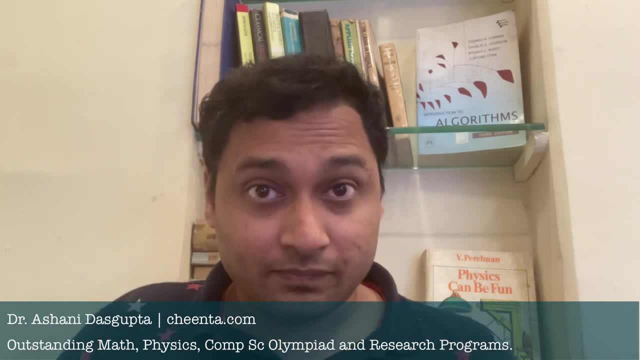 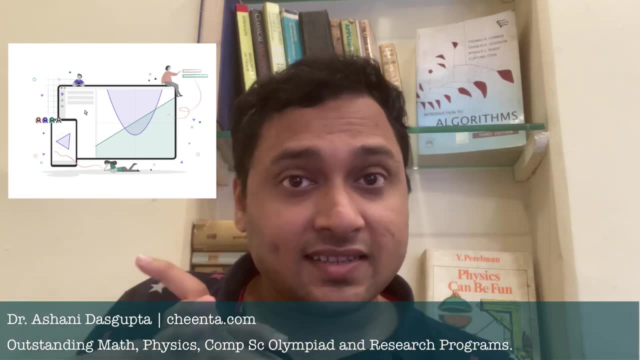 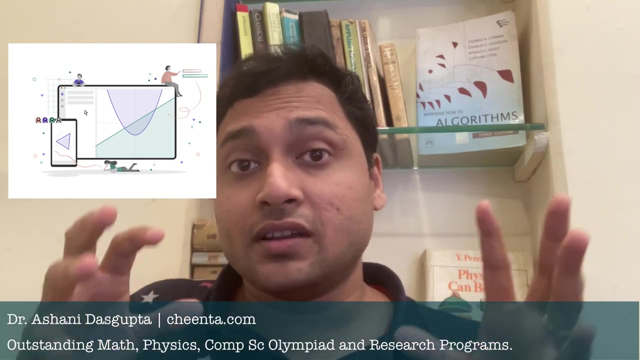 we incorporated on the way in our curriculum. We always did a little bit of computational mathematics at that level. We used tools like GeoGebra to create platonic solids like Q, octahedron, icosahedron and so on. These are very beautiful, and when you do it using GeoGebra- 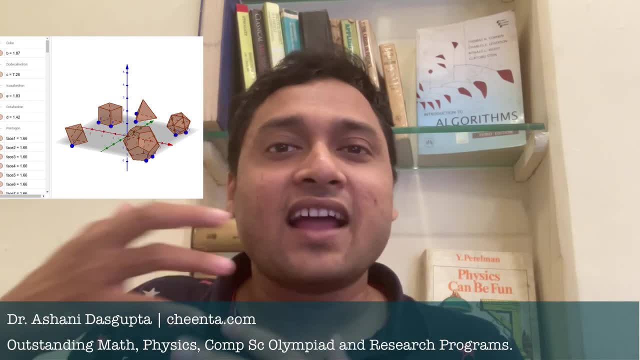 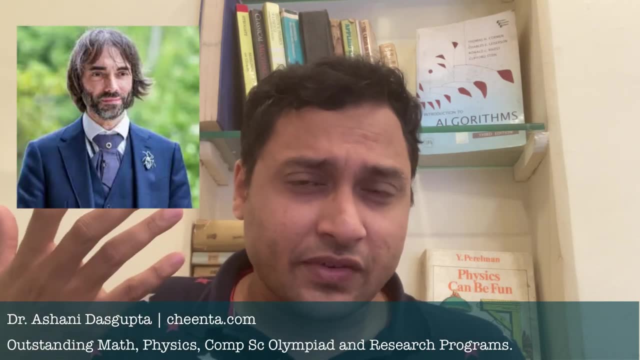 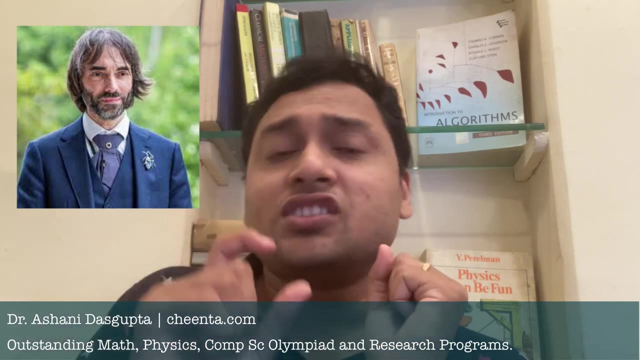 or using paper. it is a very hands-on kind of experience with mathematics and that is very helpful. In fact, one of the greatest mathematicians of our time, Cedric Villani, created a very beautiful investigation on how to teach mathematics at elementary school level. 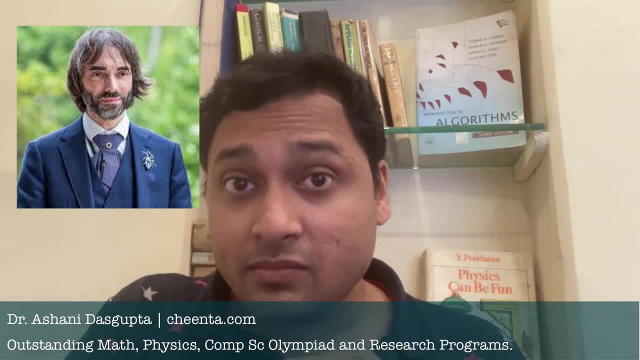 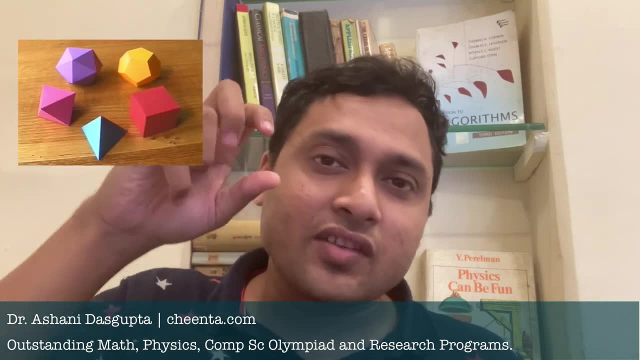 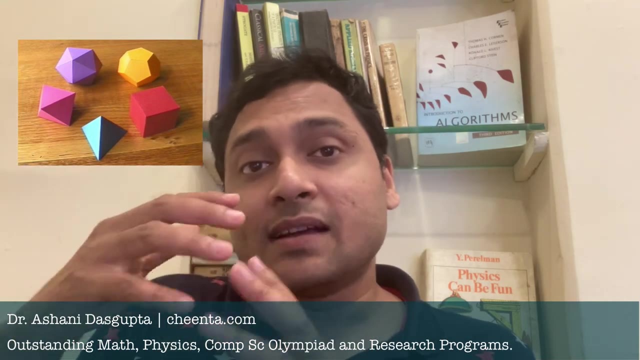 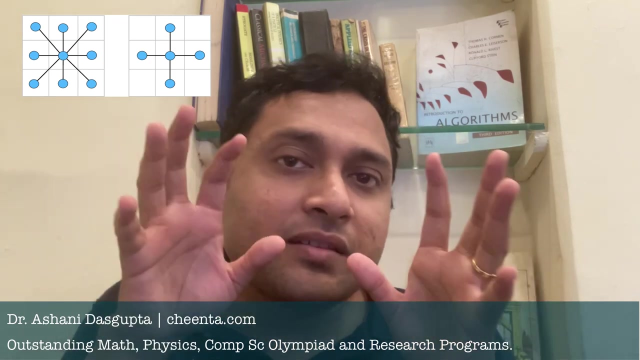 and one of his recommendations was to do hands-on mathematics. Now, having said that, with the creation of cubes and the creation of paper models of those platonic solids, we also now added something called coloring. So in mathematics, adjacency relation is a very important relation. 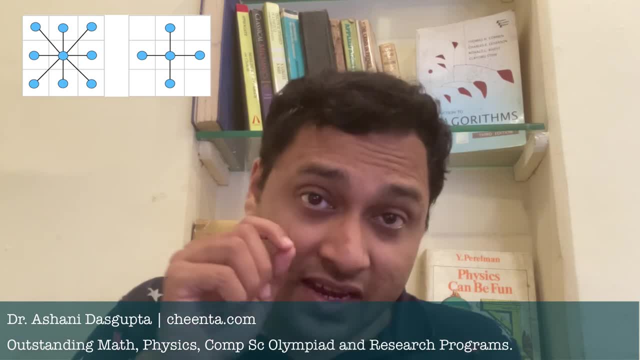 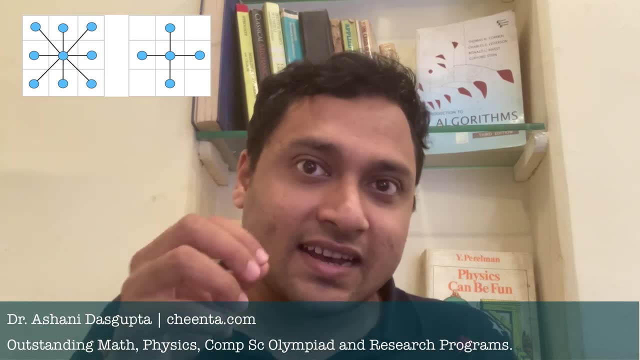 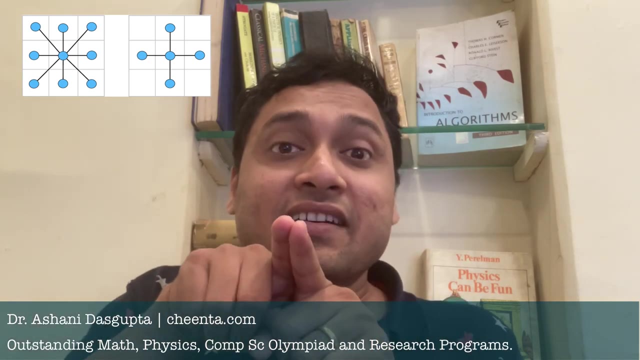 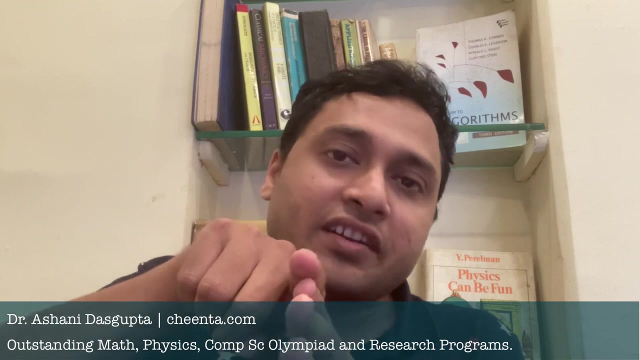 In fact, relations themselves are quite important. It's very intuitive and structured in nature to understand relation. It's sort of the first step toward understanding structured knowledge. We say two faces of a cube are adjacent if they share an edge. Two faces are adjacent if they share an edge. This is a relation that we are imposing. 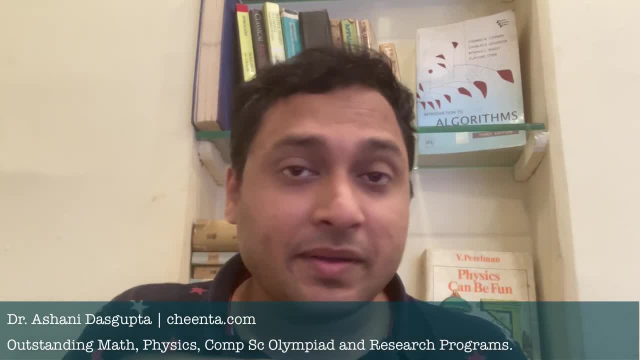 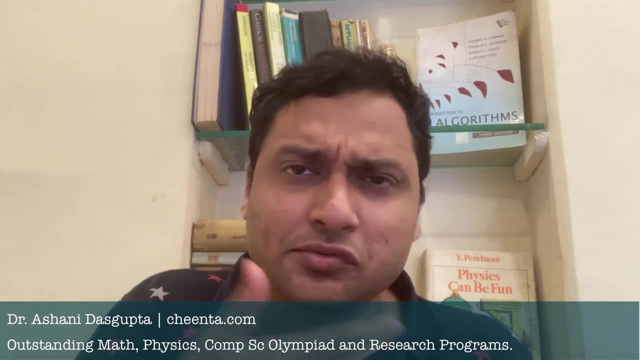 on the faces, the six faces of a cube, I mean. the same thing can be done with any other solid. Now for a young mind who is in like grade 2,, 3,, 4,, it's hard to sort of single out those pairs of. 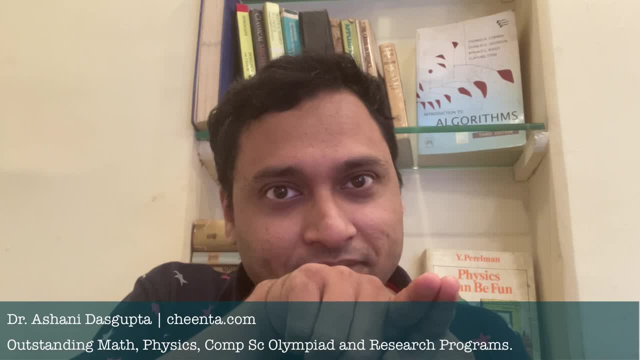 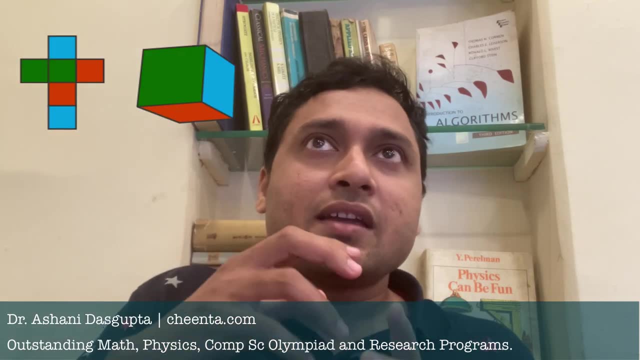 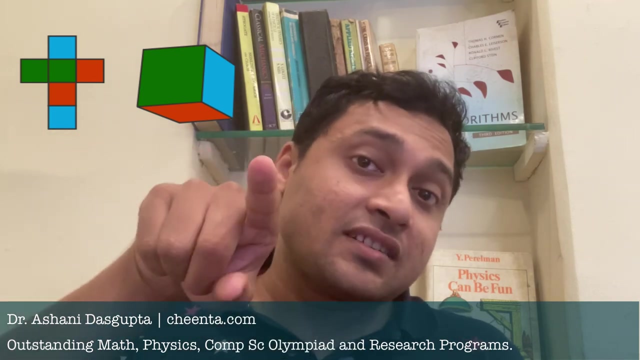 faces which share an edge. So we recently did this, We introduced something called a coloring technique. So we said, hey, color the different faces of the cube, but make sure that two adjacent faces do not have the same color. That was an interesting problem. 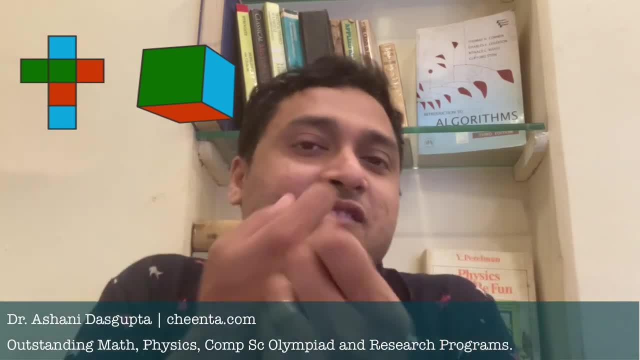 What we saw is once we were not abstractly explaining what is adjacency, but, as than to do something like a coloring, but ask them to do something like a coloring, in this sort of grasping pattern we walked through operations like a worth statement, like an extra component, like a little appointment. but ask them to do something like a coloring: compare the faces. likeabyrinth that was observed. a half gradual hindrance from the variety of faces replaced by minutes, a half gradual impression, and it's also like this always occur: lions 그�ven- την, Tennessee. or zoom in on the faces that were tomatokraftvenidos' ones. 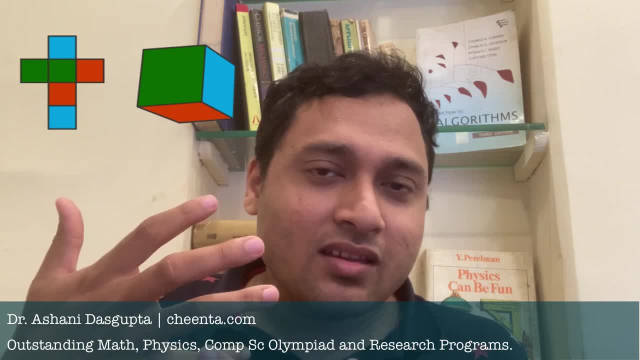 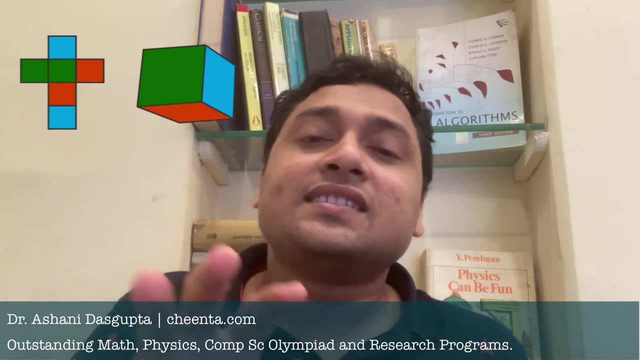 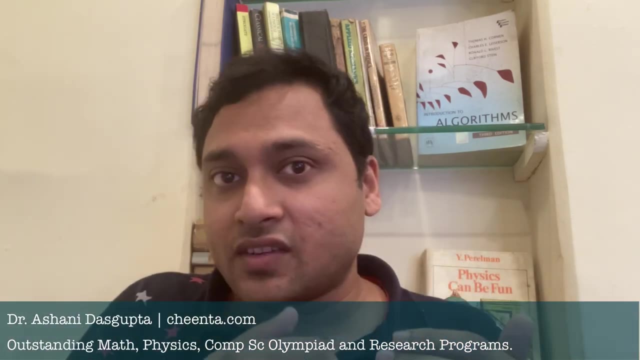 they sort of grasped the idea pretty quickly and then we could actually propose more complex problems. for example, we could say: what is the minimum number of different colors? you need to do such a thing to color the faces of the cube, with adjacent faces having distinct colors. 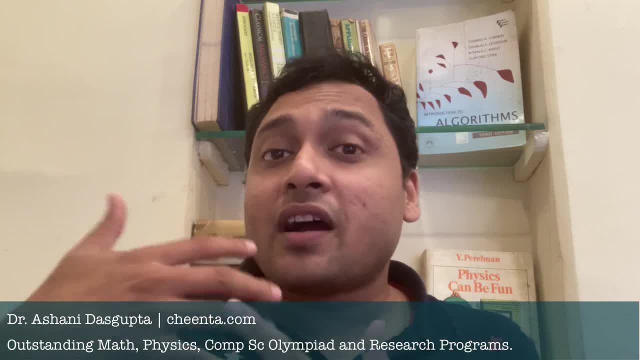 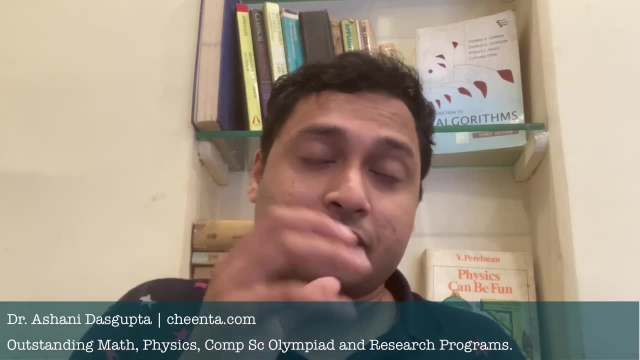 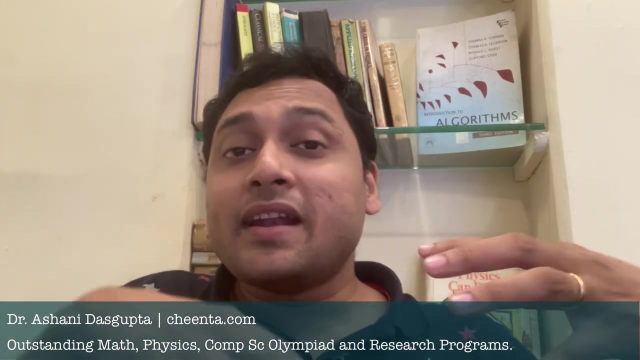 we asked another question which was a little bit more complicated. if you want to do different colorings of the cube and you are not, different means two colorings are different. if you turn the cube you cannot convert one coloring into another. so how many different colorings of the cube are? 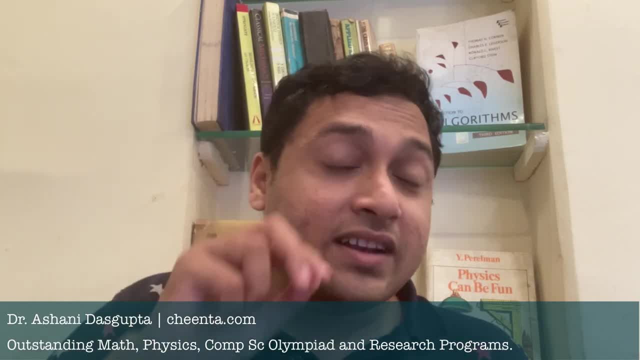 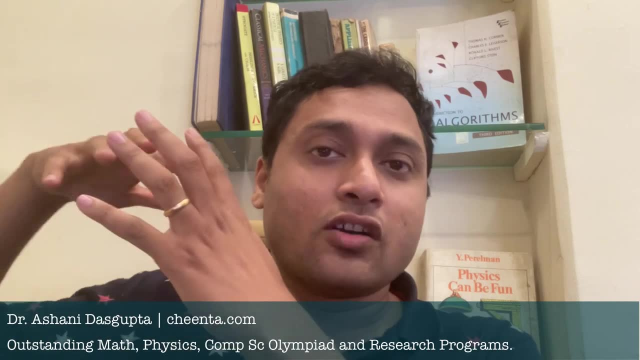 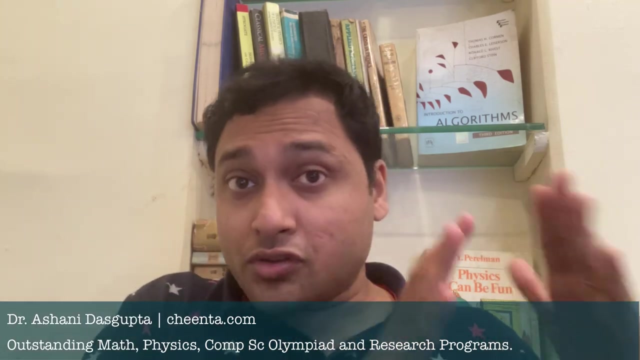 possible, such that two adjacent faces do not have the same color. so we did it for the cube, we did it for other platonic solids like icosahedron, octahedron and so on, and second graders, third graders, fourth graders. really we did not do it with the first grade. 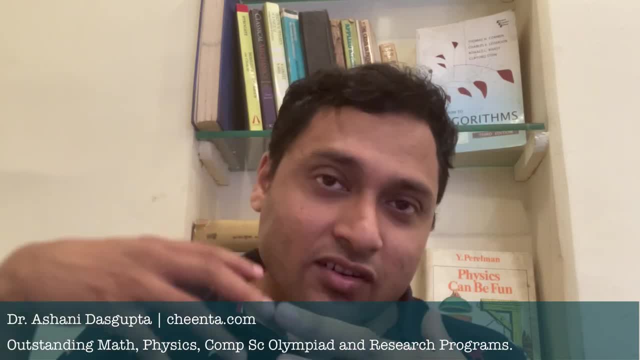 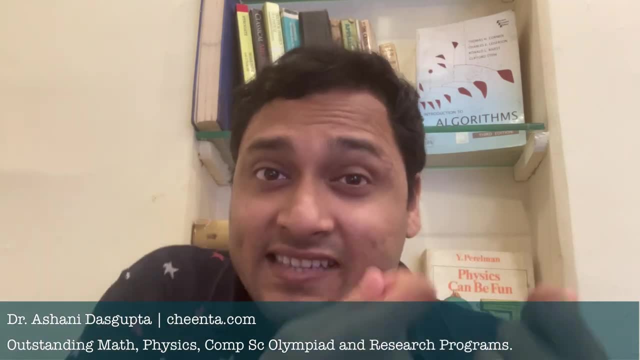 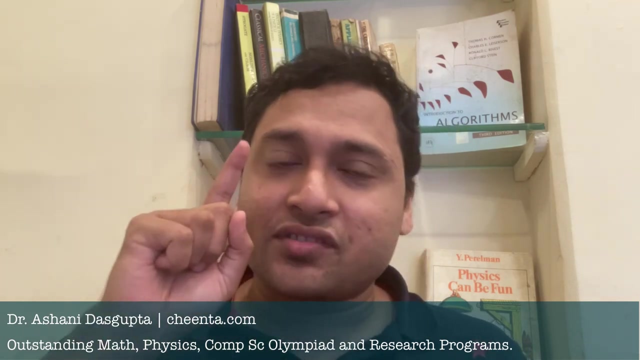 we did it with the second grade, spin and, and these three graders, uh, they could understand and they could actually. we see, we saw that they were involved in the process of actually coloring it, actually guessing what the answer is, trying to recognize some sort of a pattern. 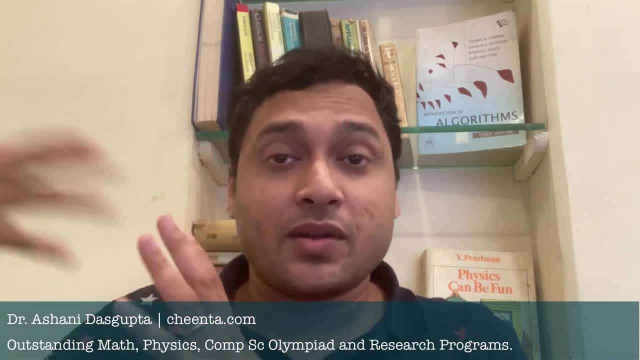 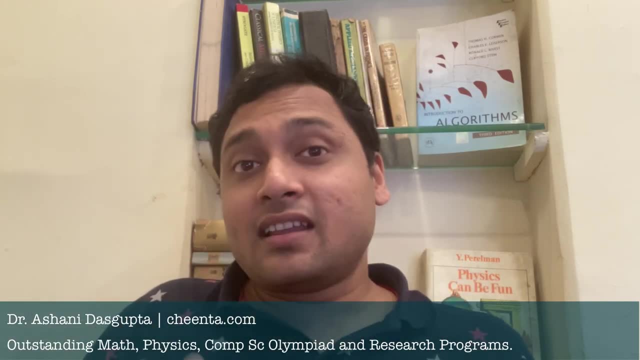 it's a very interesting exercise. you can try this in your home and with your children, or if you have a brother or sister who wants to try some nice mathematics, you can also do that. that we are still learning. even after 10-12 years of doing this, we are still. 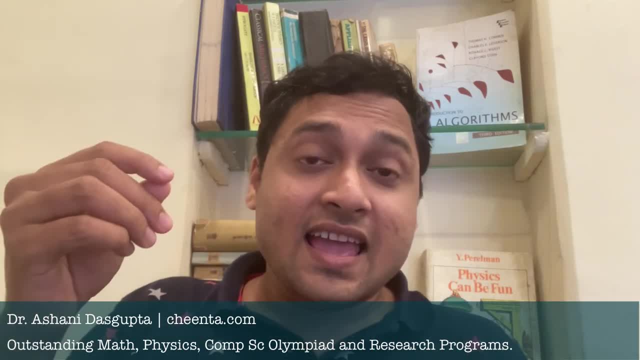 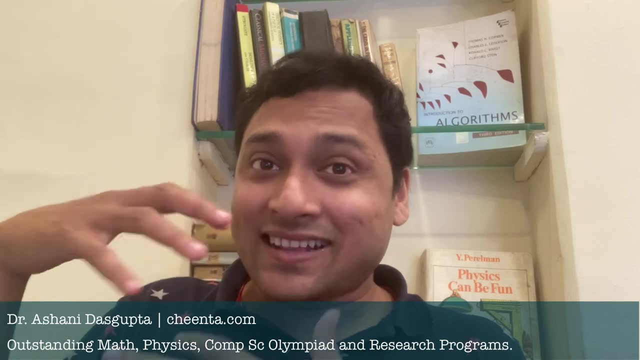 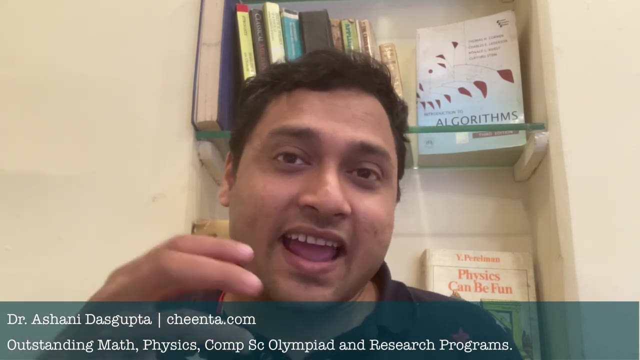 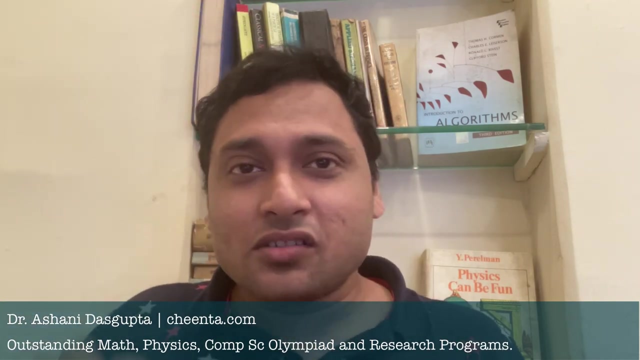 learning how to teach mathematics effectively at that stage, the stage of elementary school. it's a very interesting exercise for us as teachers: how to develop a nice curriculum that provoked interest and energizes the student and creates a foundation for a long-term mathematical journey. so it's 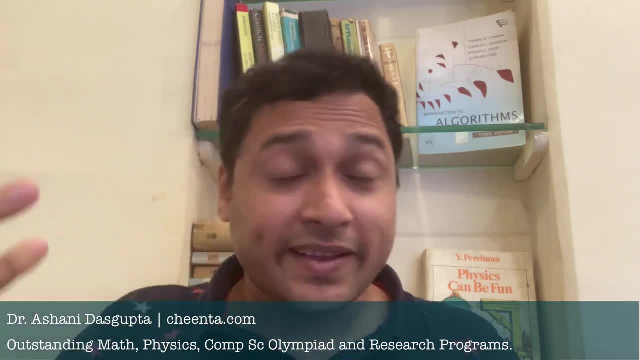 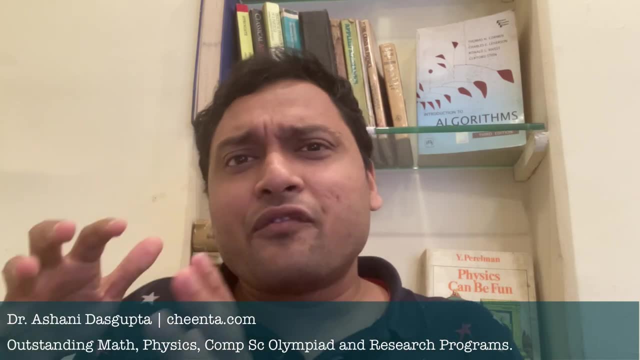 a hard work. if you have ideas, please put them in the comment. if you have questions, please put them in the comment, and we are very glad to discuss these things with each other. we have whatsapp groups where we discuss these things. you can go to cintacom link in the description and join us via whatsapp.